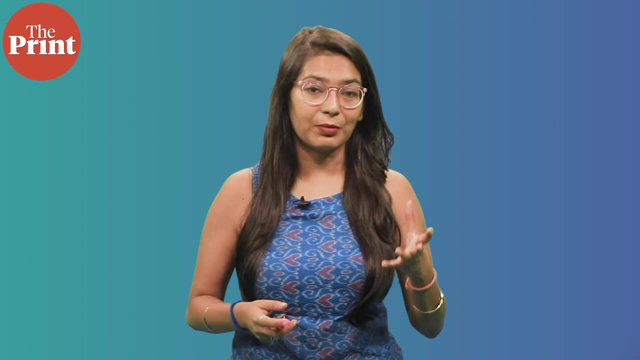 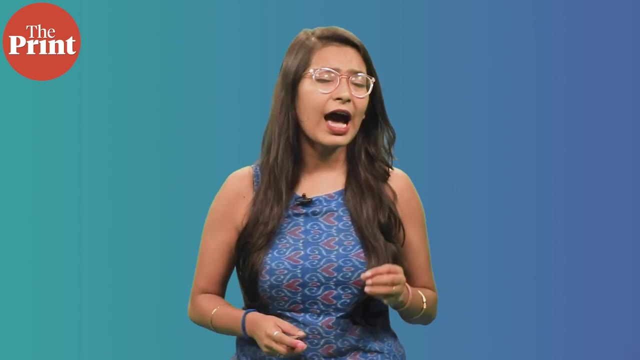 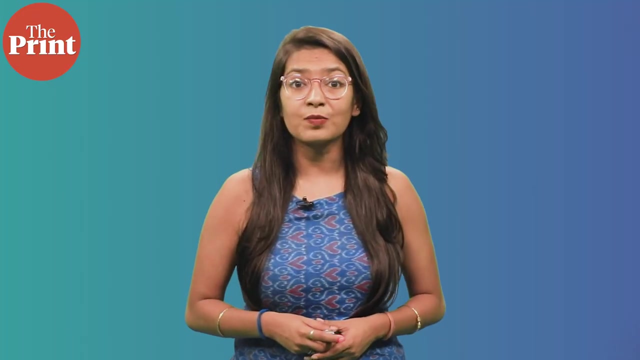 on Earth, But not all the birds alive at the time made it. Why the ancestors of modern birds lived while so many of their relatives died has been a mystery that paleontologists have been trying to solve for decades Now. two new studies point to one possible factor. 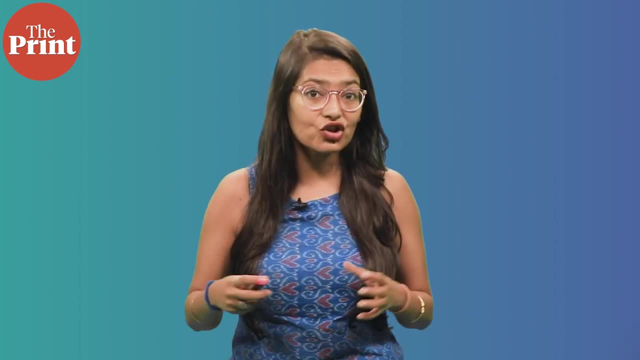 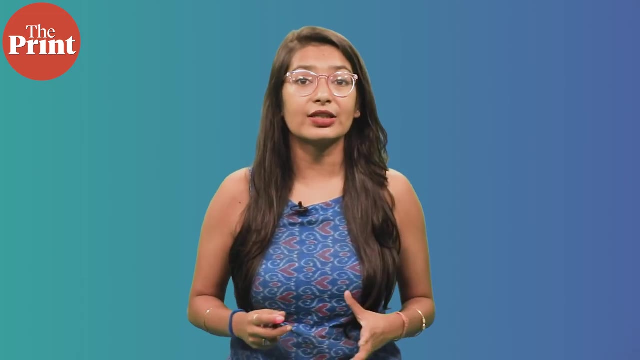 the differences between how modern birds and their ancient cousins molted, that is, shed and regrew their feathers. In this episode, I tell you all about molting, what the new studies have found and why it is an important piece of history. 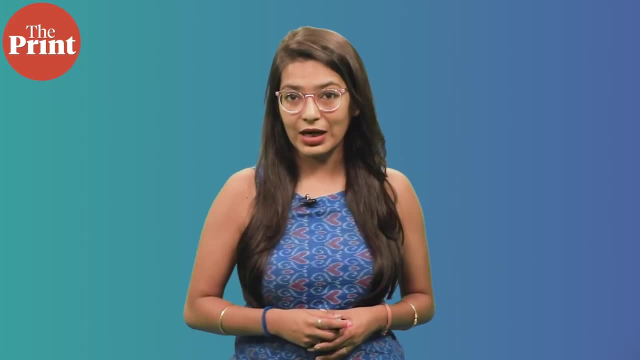 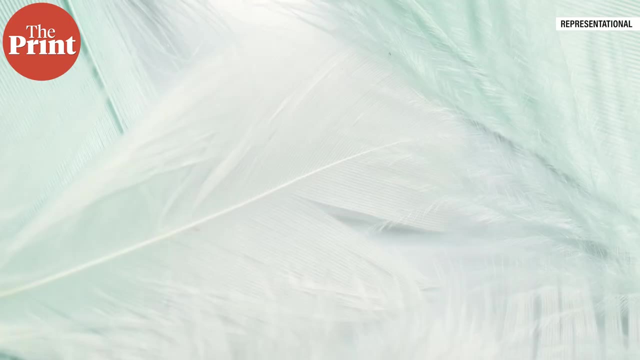 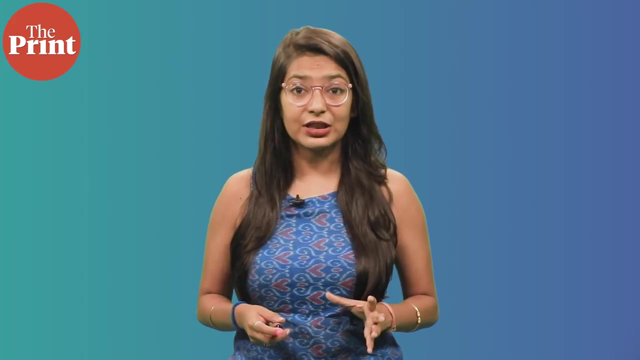 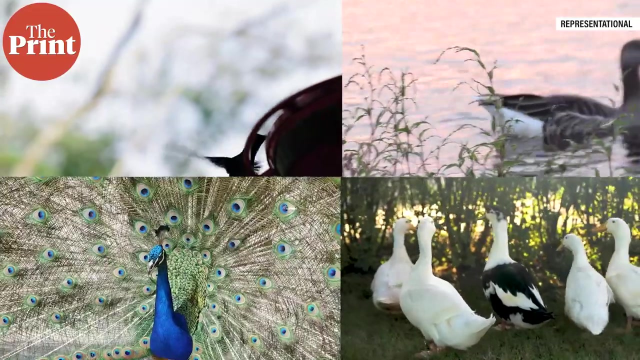 Feathers are one of the key traits that all birds share. They are made of a protein called keratin, the same material as our fingernails and hair, And birds rely on them to fly, swim, camouflage, attract mates, stay warm and protect against the sun rays. 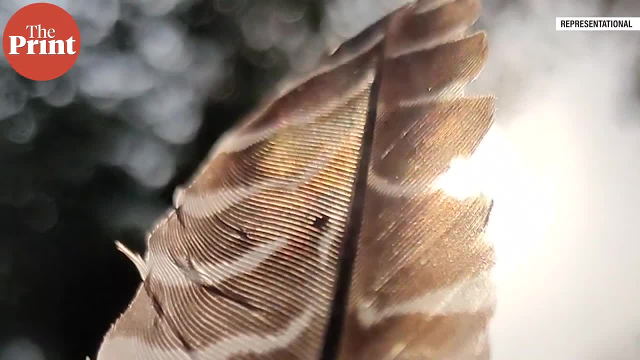 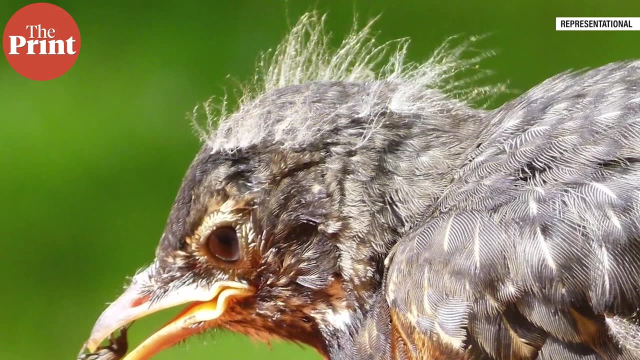 But feathers are not the only thing that has changed in the history of evolution. In the past, there were complex structures that can't be repaired, So, as a means of keeping them in good shape, birds shed their feathers and grow replacements. This process is called molting. Baby birds molt in order to lose their baby feathers and grow adult ones. Mature birds continue to molt about once a year. At some point in our lives we have found ourselves collecting a stray bird feather, According to researchers from the Chicago. 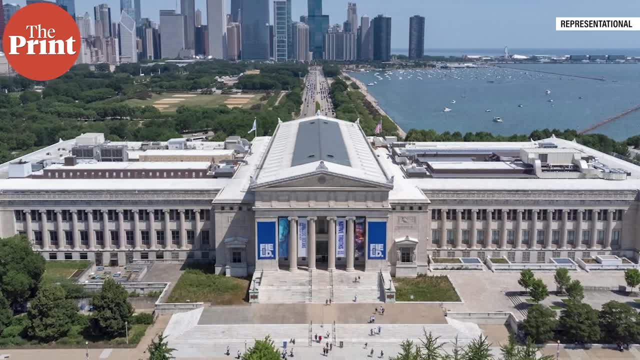 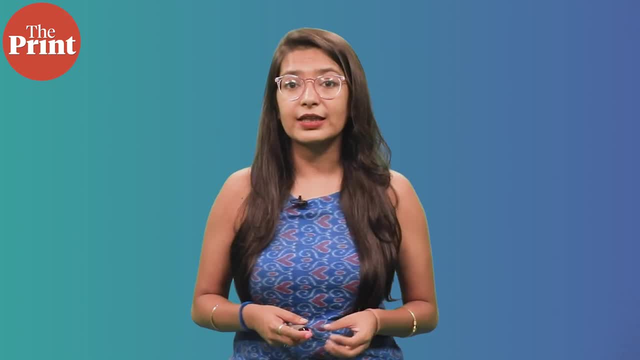 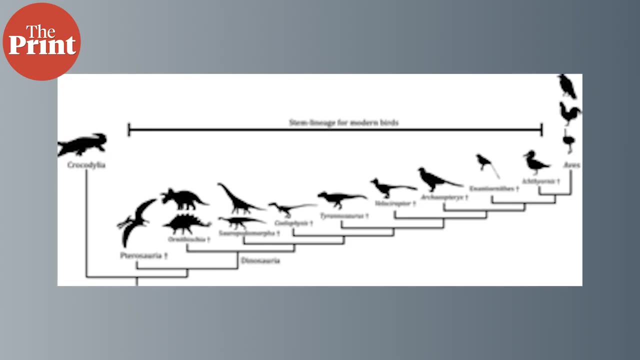 Field Museum. molting is a fundamentally important process to birds because feathers are involved in so many different functions. The team wanted to find out how did this process evolve, how it differed across groups of birds and how it shaped bird evolution. Two new studies have examined the molting process in prehistoric birds. 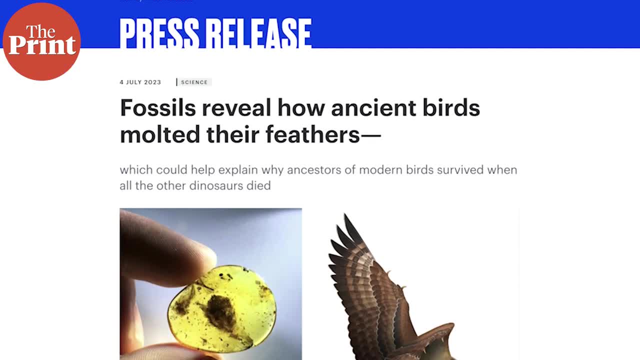 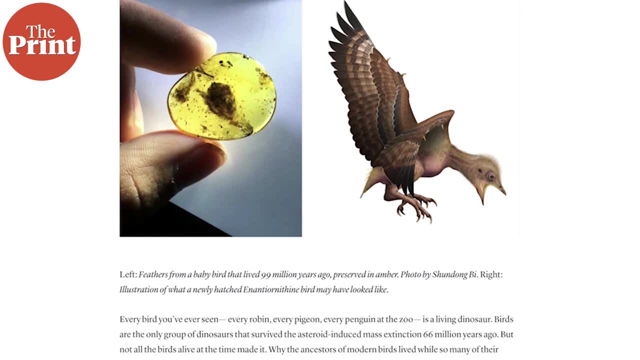 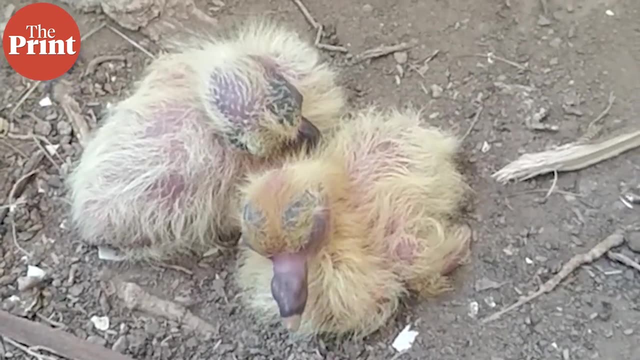 The first paper in the journal Cretaceous Research detailed the discovery of a cluster of feathers preserved in amber from a baby bird that lived 99 million years ago. Today, baby birds are on a spectrum in terms of how developed they are when they are born and 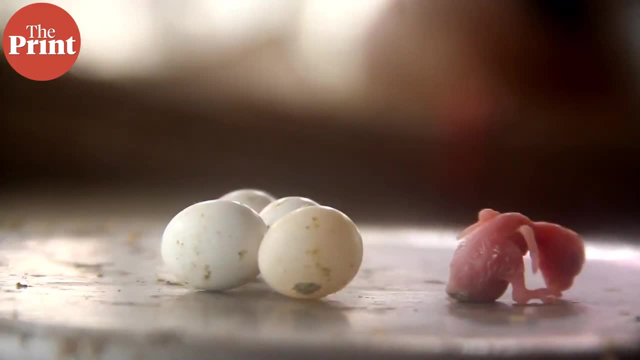 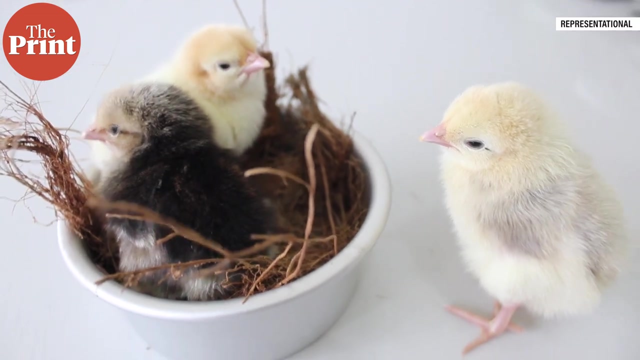 how much help they need from their parents. Altishield birds hatch naked and helpless. They lack the feathers, which means that their parents can more efficiently transmit body heat directly to the baby's skin. On the other are born with feathers and are fairly self-sufficient. All baby birds go through. successive moulds periods. when they lose feathers, they have and grow in a new set of feathers before eventually reaching their adult plumage. Moulding takes a lot of energy and losing a lot of feathers at once can make it hard for the bird to keep itself warm As a result. 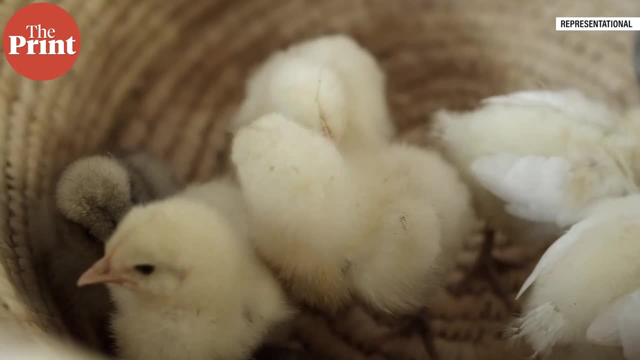 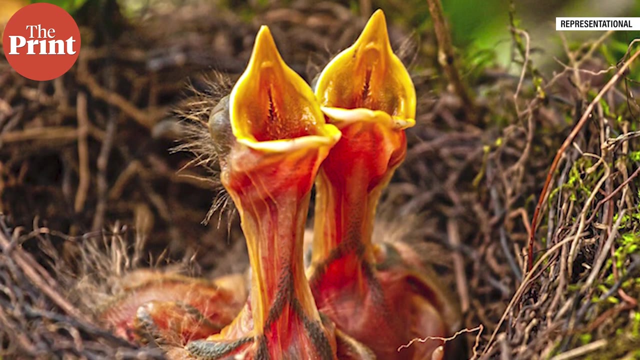 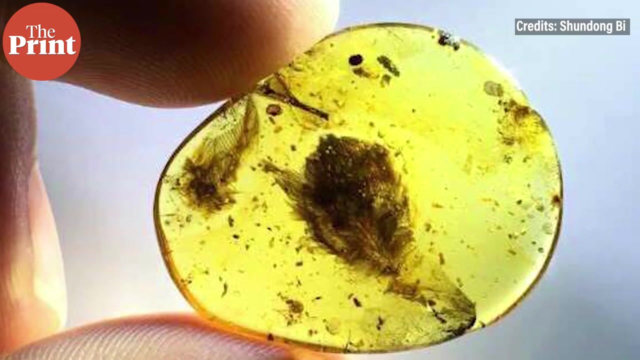 precocial chicks tend to mould slowly so that they keep a steady supply of feathers, while altricial chicks that can rely on their parents for food and warmth undergo a simultaneous mould that is losing all their feathers at roughly the same time. The amber preserved feathers in this. 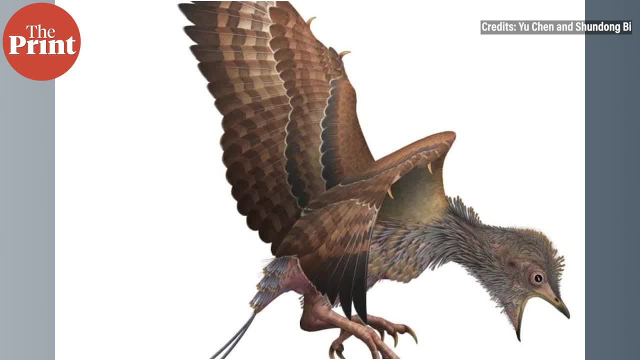 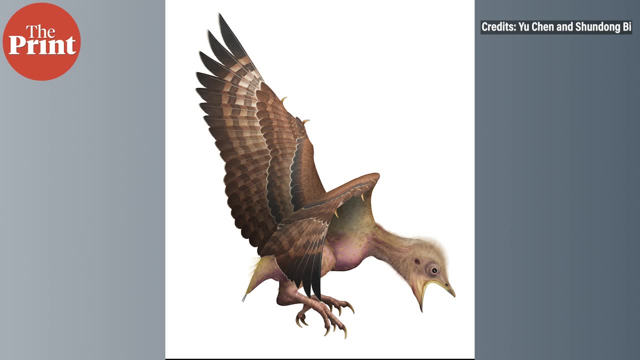 study are the first definitive fossil evidence of juvenile moulding, and they reveal a baby bird whose life history does not match any birds alive today. The speciality of the precocial chicks is that they have a lot of feathers and they have a lot to learn. The specimen is combination of precocial and altricial characteristics. According to the 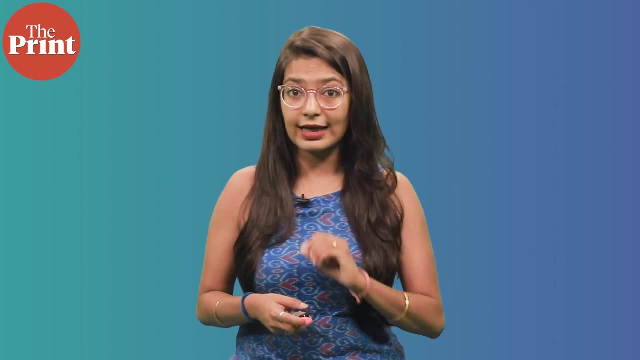 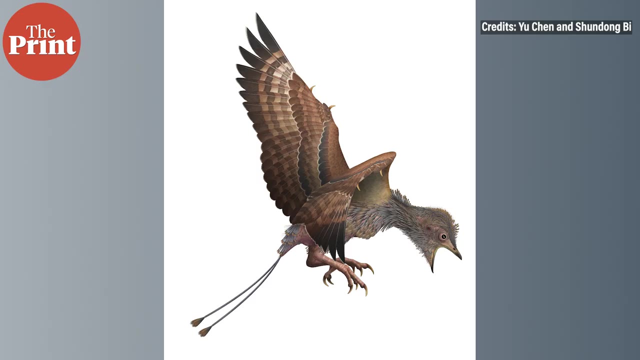 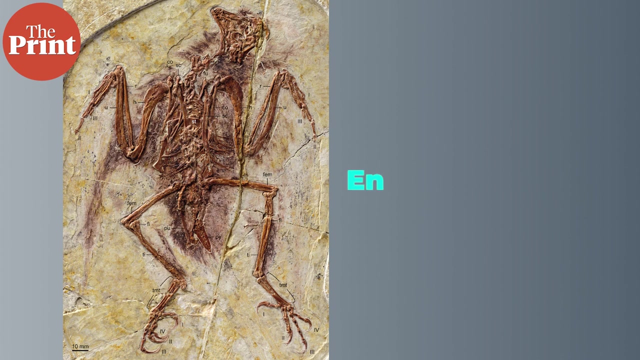 researchers, all the body feathers are basically at the exact same stage in development, So this means that all the feathers started growing almost simultaneously. However, this bird was almost certainly part of a now extinct group which is called Enantiornithinus, which were 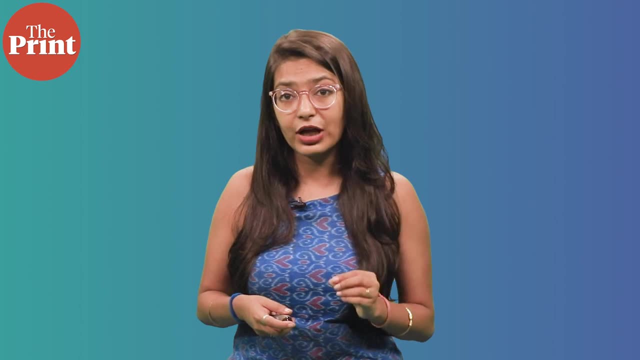 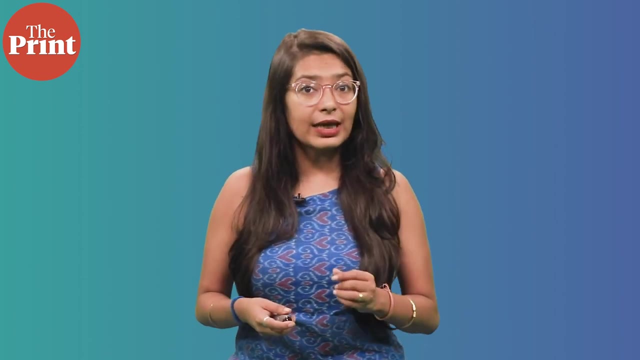 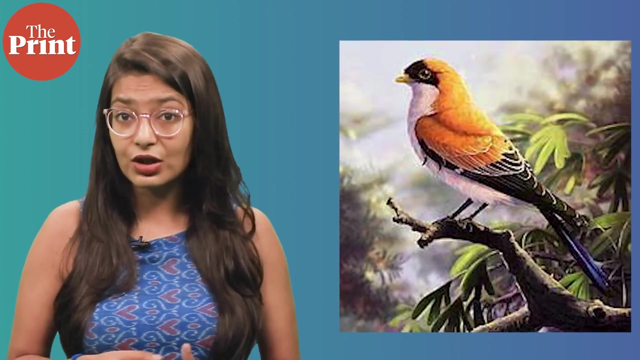 highly precocial. The researchers hypothesized that the pressures of being a precocial baby bird that had to keep itself warm while undergoing a rapid mould might have been a factor in the ultimate doom of these birds. During the Cretaceous period, this species was the most diverse group of birds, but they went extinct along with the other non-avian dinosaurs. When the asteroid hit, global temperatures would have plummeted and resources would have become scarce. So not only would these birds have even higher energy demands to stay warm, but they didn't have the resources to meet them. Meanwhile, another study published in the journal 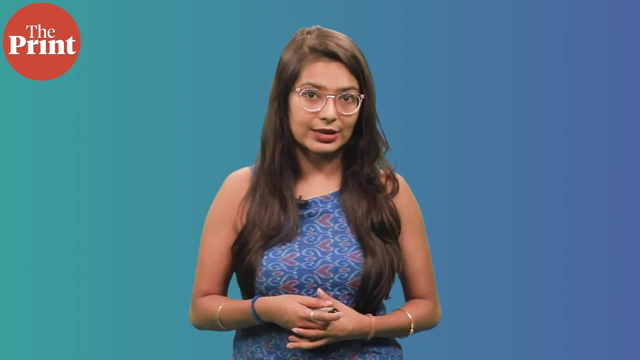 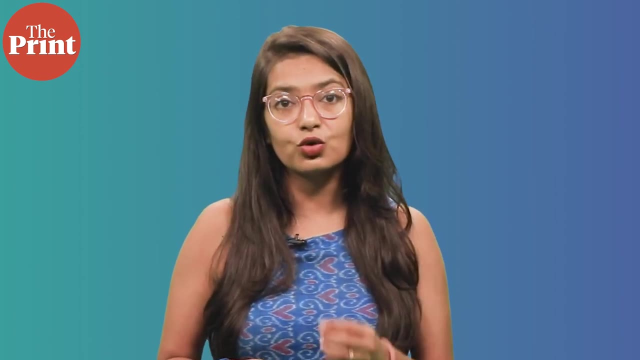 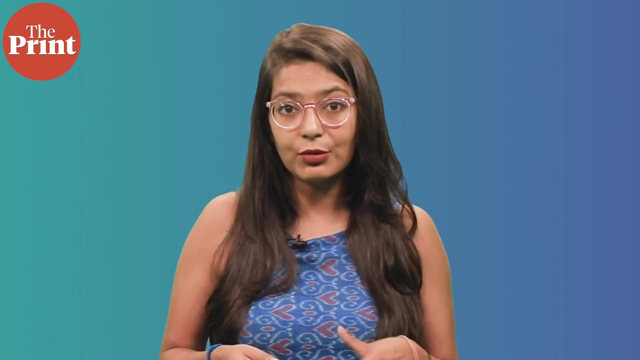 Communications Biology examined moulding patterns in modern birds to better understand how the process first evolved. In modern adult birds, moulding usually happens once a year in a sequential process in which they replace just a few of their feathers at a time over the course of a few weeks. That way, they are still able to fly throughout the moulding process. 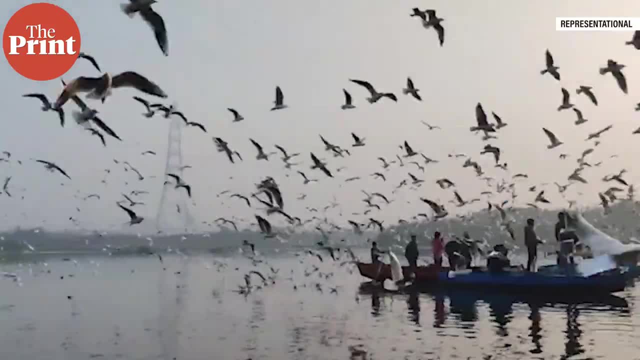 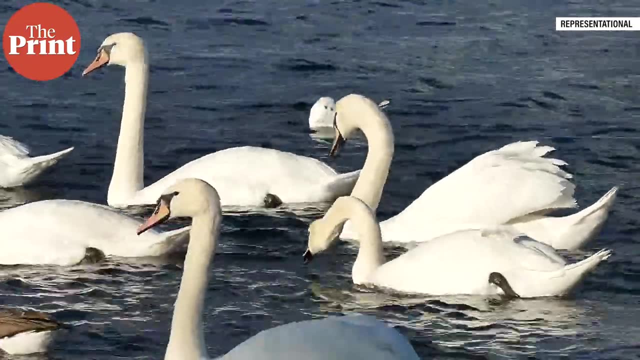 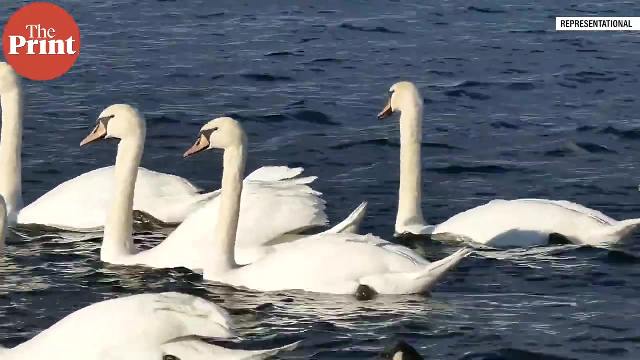 Simultaneous moulds in adult birds, in which all the flight feathers fall out at the same time and regrow within a couple of weeks, are rarer and tend to show up in aquatic birds like ducks that don't absolutely need to fly in order to find food and avoid predators. It's very rare to find. 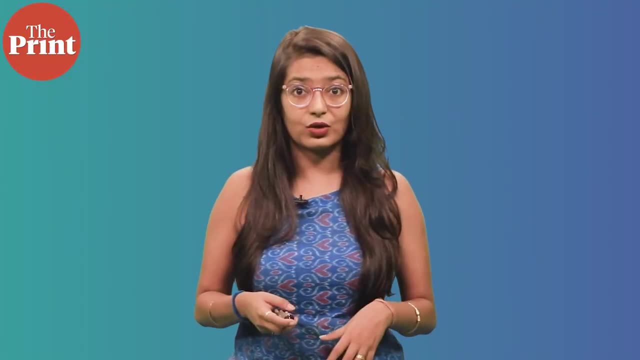 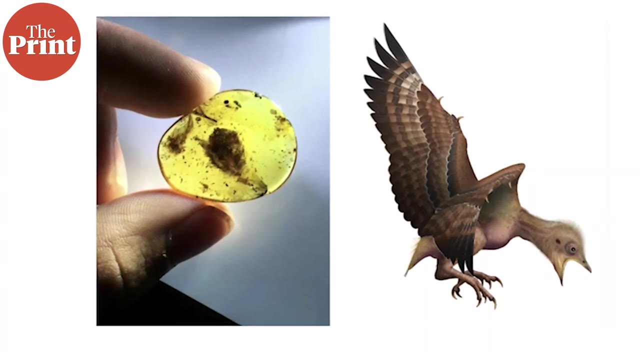 evidence of moulding in fossil birds and other feathered dinosaurs, but researchers so far did not know why. The thought was that birds with simultaneous moulds which occur in a shorter duration of time will be less represented in the fossil record because less time is spent moulding.